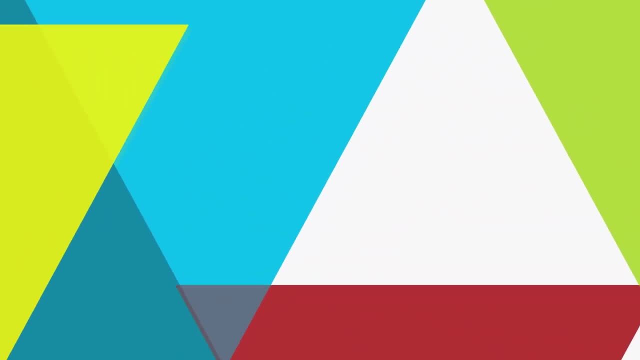 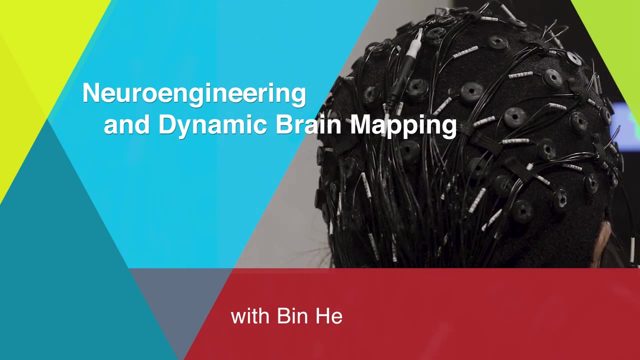 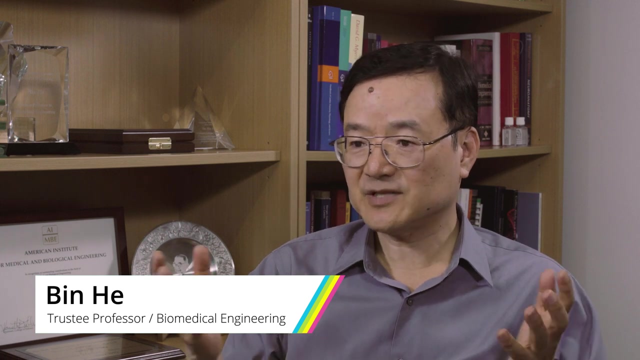 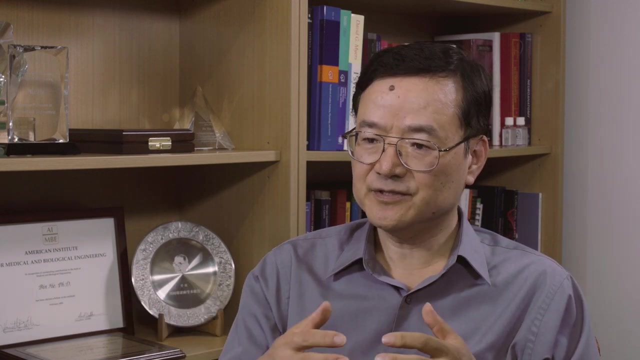 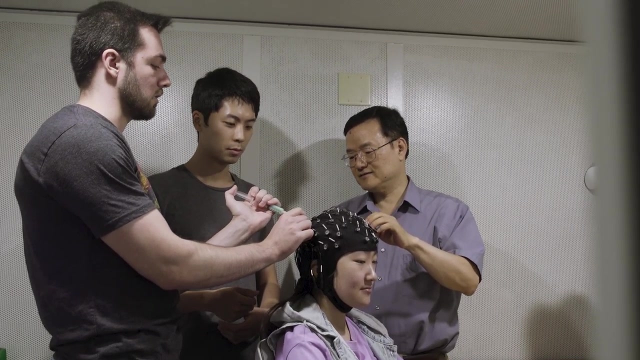 I'm working on broadly in the field of neuroengineering and recently we are focusing on developing a novel dynamic brain imaging technology, or sometimes called functional neuroimaging, And different than the functional MRI or other imaging modality is we use electromagnetic signal, so we put a cap over the scalp to record a multi-channel electrical signal. 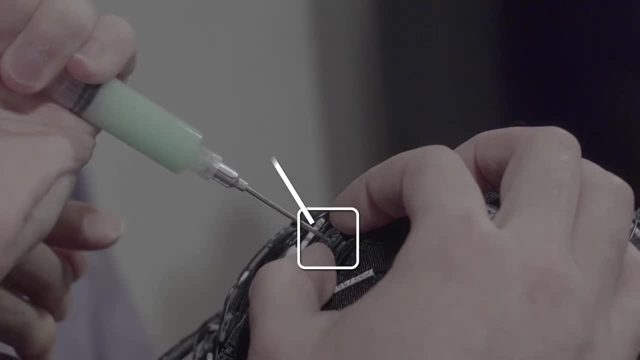 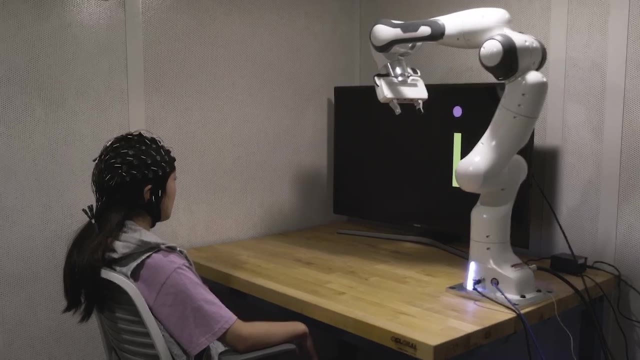 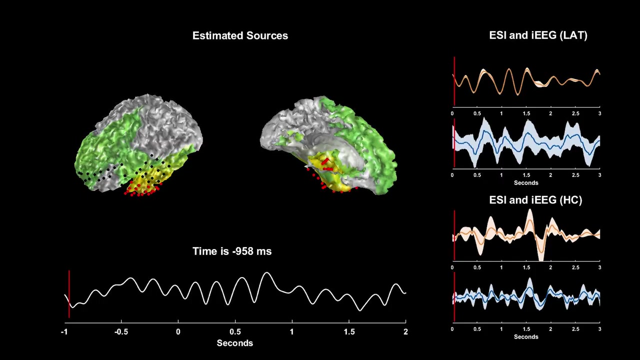 It could be magnetic signal reflecting dynamic, instantaneous and brain activation, And from there our innovation is to develop a machine learning and signal processing algorithm so we can project back from surface of the scalp and to inside of the brain to show that how three-dimensionally, how the neuro information processing propagation is going to be occurring. 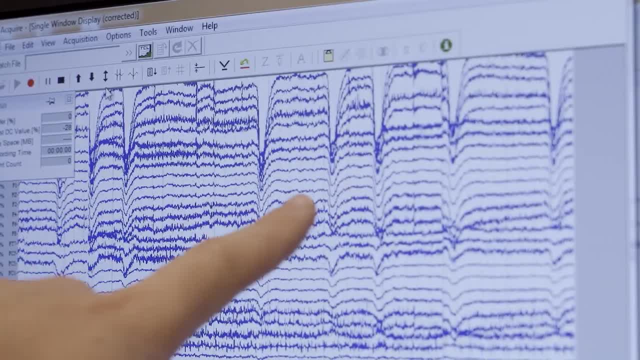 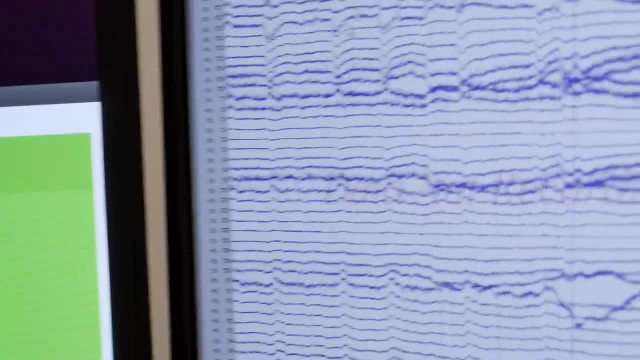 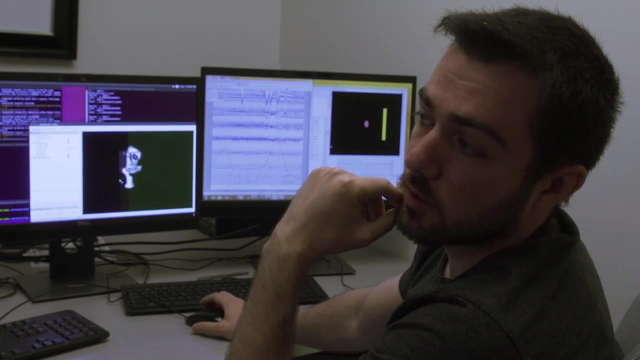 To understand how the cognition, perception and the various motor function and, most importantly, it has important clinical application, such as in epilepsy or depression or pain, or in various neurological and mental disease. The impact of this work, I think, has two-fold. 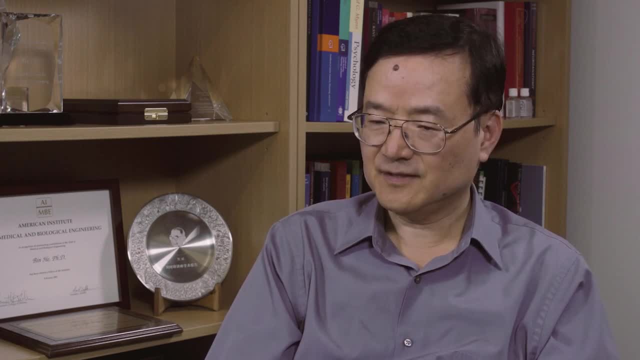 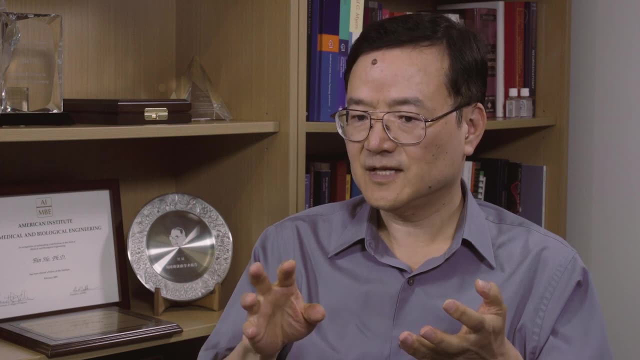 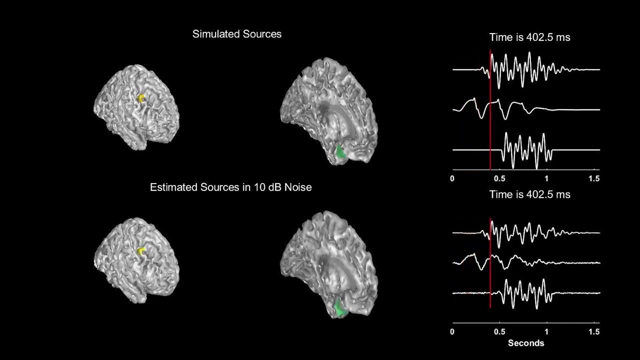 One is to establish a fundamental technology That is in the neuroimaging we all know CT, PET, MRI are all there, but all of these technology cannot provide high spatial and temporal resolution imaging of the brain function. Our technology is aiming at become one outside. the doctor can prescribe from a array of electromagnetic 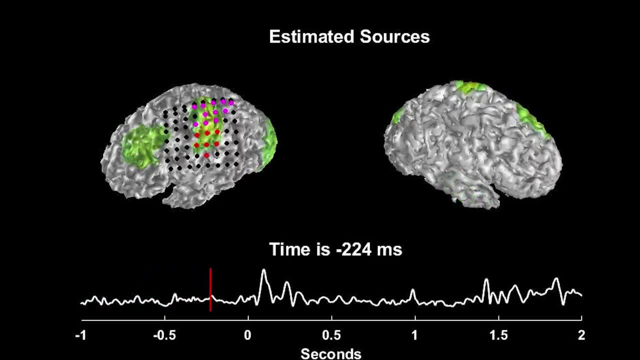 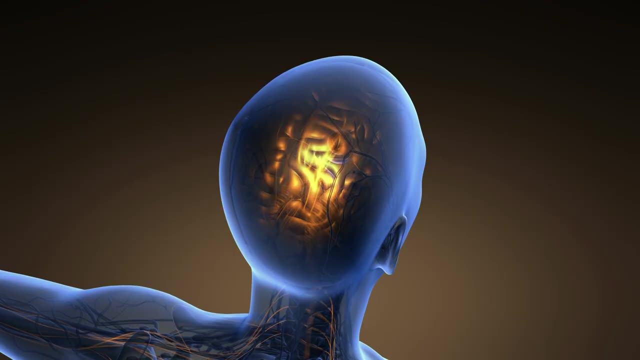 recording To provide a dynamic brain pictures. There are many disease. for example, we look into stroke, we look into pain and, most importantly, we look into epilepsy, a disease that impacting 70 million people in the world. So if this technology eventually fully develop, it could make the epilepsy surgery into potentially. 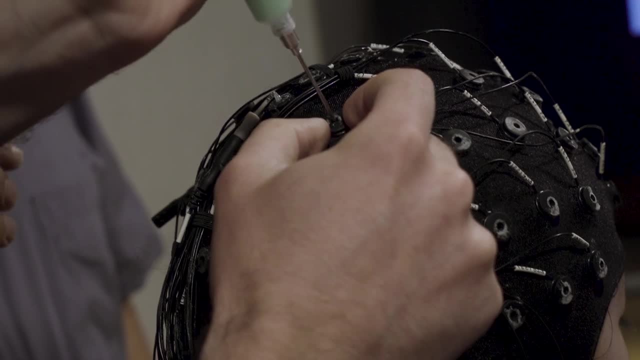 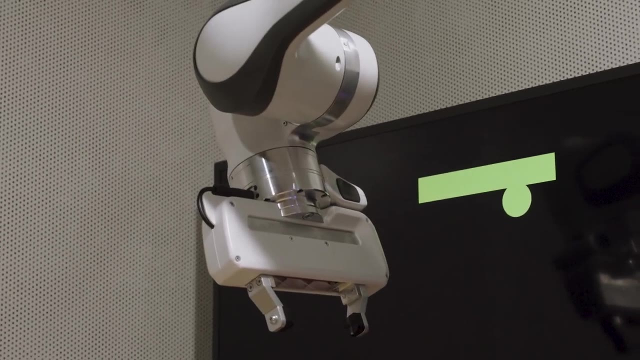 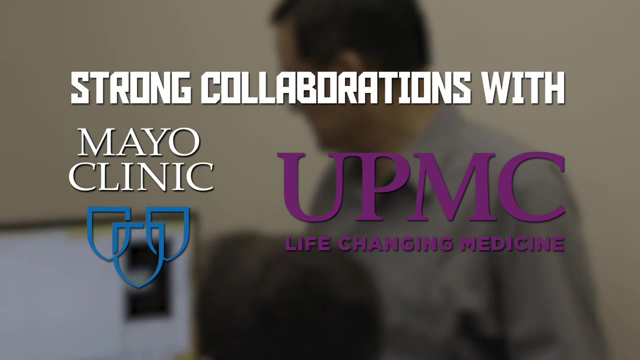 in one day. We are not just working on mass or signal processing or machine learning algorithm alone. We are solving a real problem And therefore it's really highly interdisciplinary work And we are very fortunate to have very strong collaborator at Mayo Clinic.